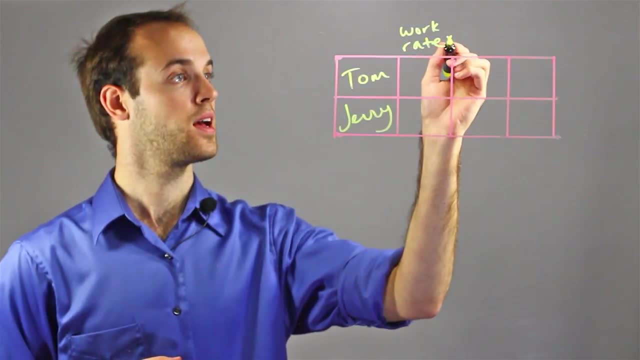 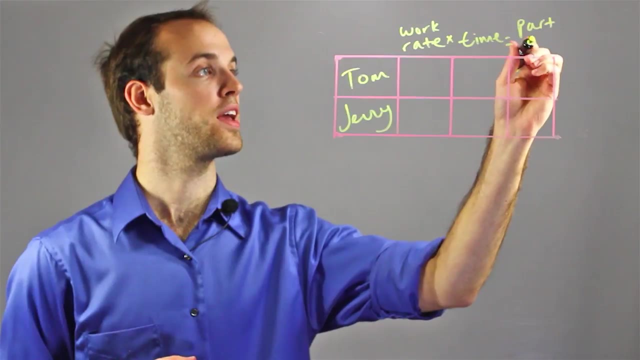 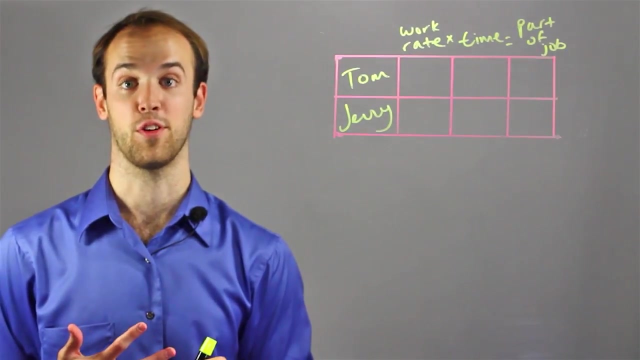 Which is how fast they work, times the time that they work, and that's going to equal the part of job that they complete. So again, Tom's work rate was one car in every 45 minutes, So his work rate will be represented by 1 over 45.. 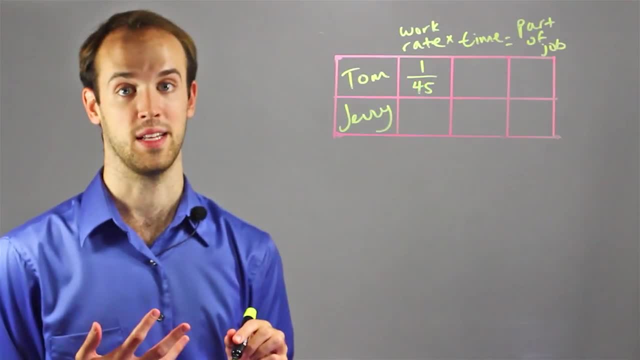 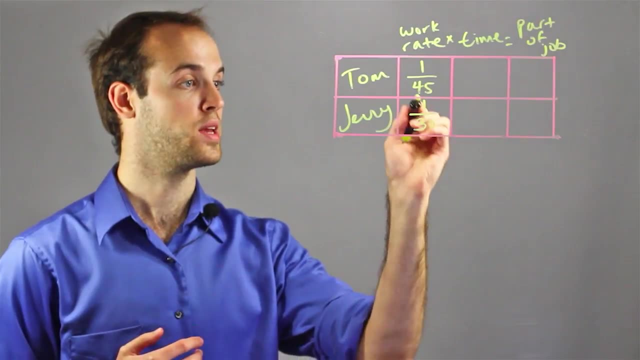 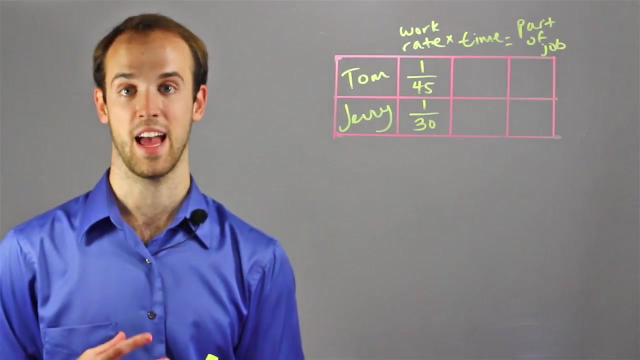 One car per every 45 minutes. Per usually means divided by. Jerry goes faster and he can do one car in every 30 minutes, So he's 1 over 30. The time is the unknown, because I want to know how fast it takes them washing the same car together. 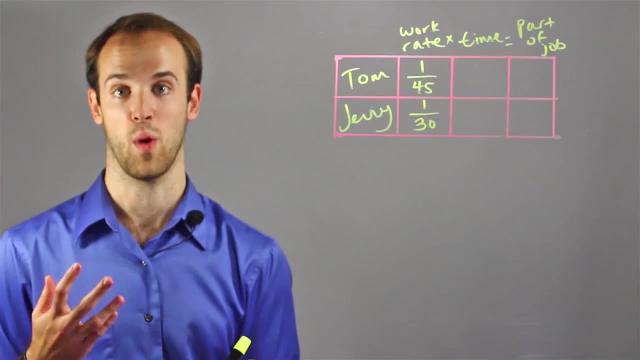 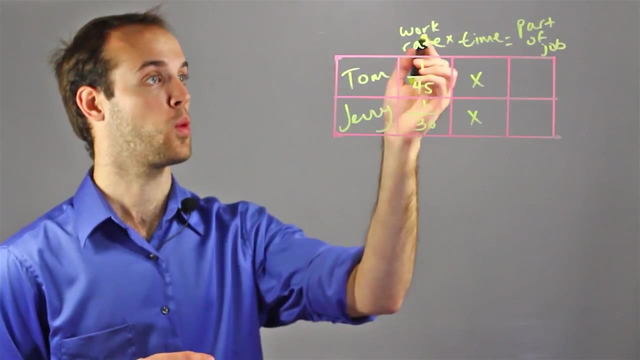 And they're going to work the same amount of time. It's not like Jerry's going to quit halfway through the job. They're both going to be represented by X And since I know that work rate times, time equals the part of the job. 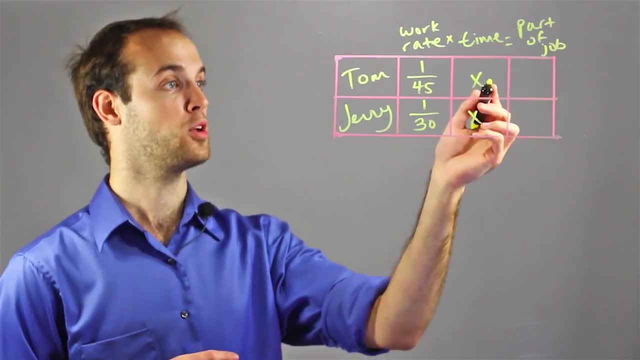 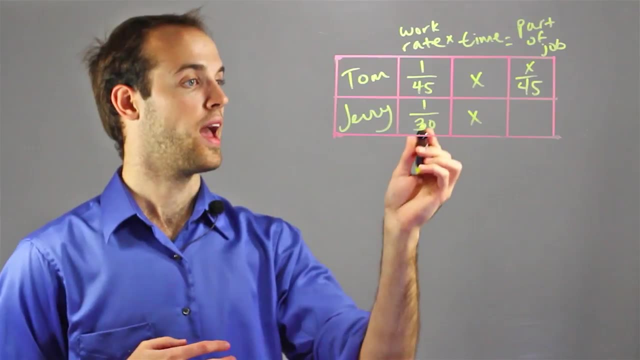 I know that I can get the part of the job column just by multiplying these two together. So X times 1 over 45.. 45 is equal to X over 45. And X times 1 over 30 is equal to X over 30.. 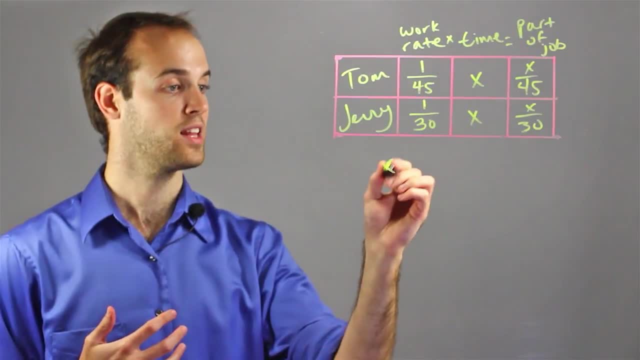 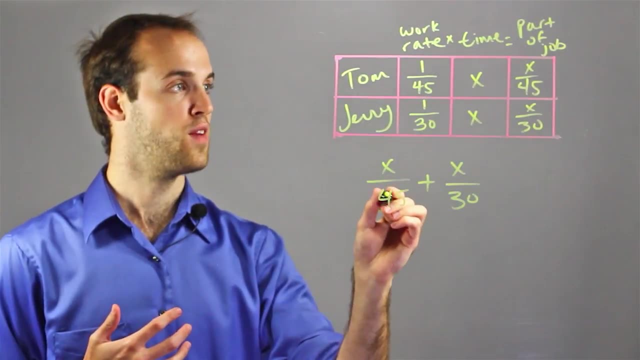 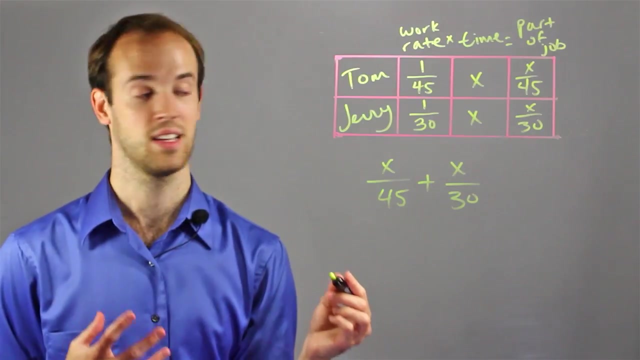 And now I'm ready to set up my equation, And I can get that just by adding the two parts of the job completed together, So X over 45, the part of the job that Tom completes plus X over 30, the part of the job that Jerry completes. 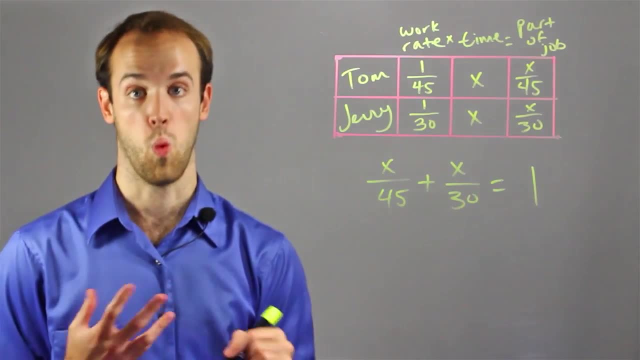 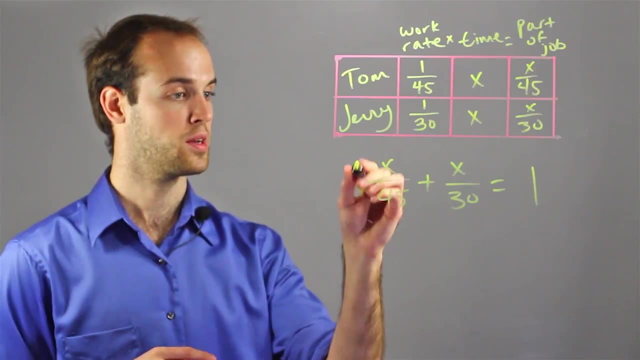 needs to be equal to 1.. 1 job: 1 job completed. 1 total job completed by both of them. So now I just have to solve this equation for X. The first thing I'm going to do is multiply both sides by 90.. 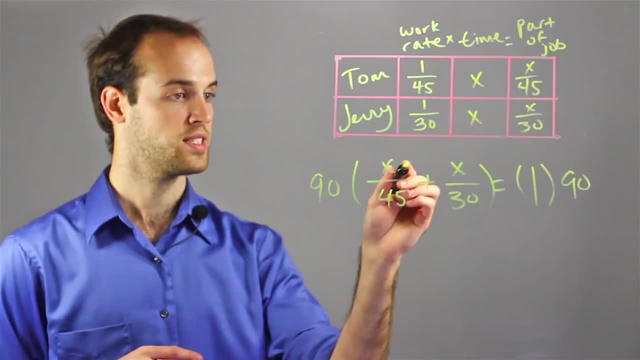 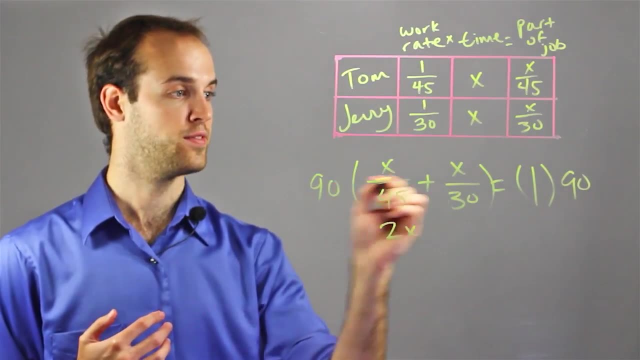 Because that will get rid of all my fractions. So on this side I would have 90X over 45,, which would simplify to 2X, And in this term I'm going to have 90 times X over 30,, which is going to simplify to 3X. 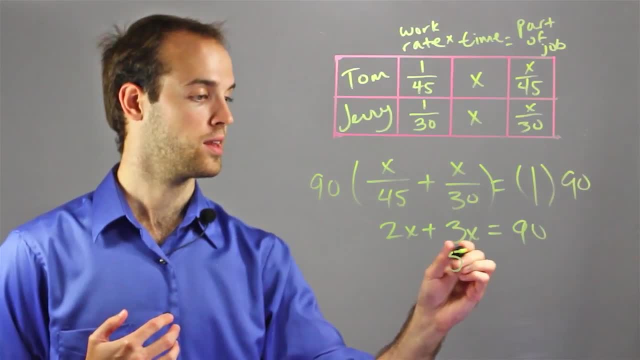 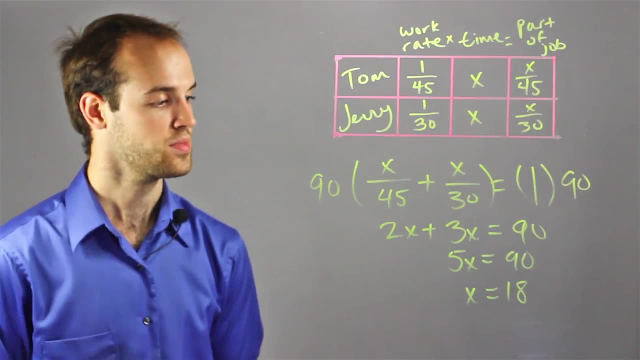 And that equals 90 times 1,, which is 90. And then combine like terms: I have 5X equals 90. And then divide both sides by 5 and I have X equals 18. So I can now determine that, Tom and Jerry, if working together will wash one car in. 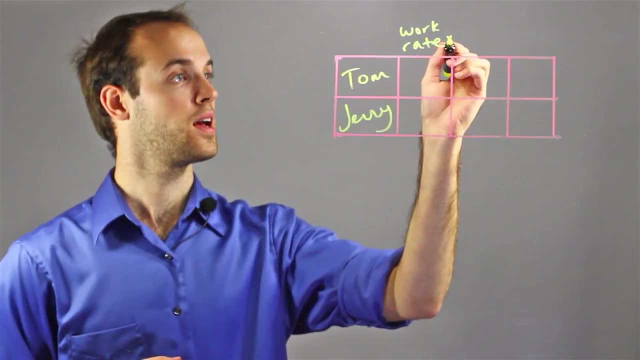 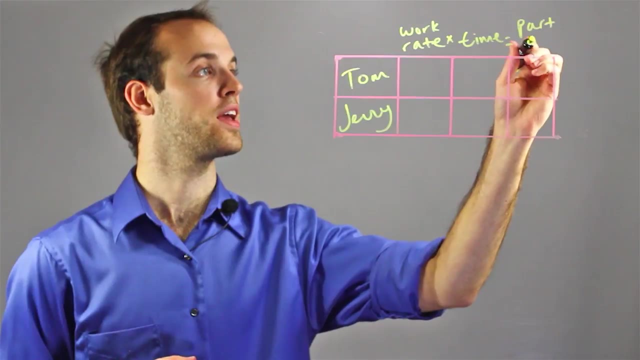 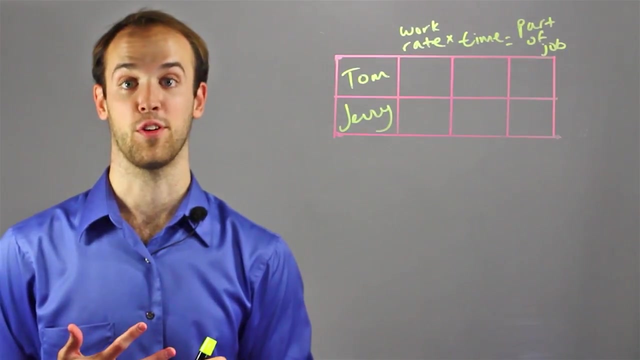 Which is how fast they work, times the time that they work, and that's going to equal the part of job that they complete. So again, Tom's work rate was one car in every 45 minutes, So his work rate will be represented by 1 over 45.. 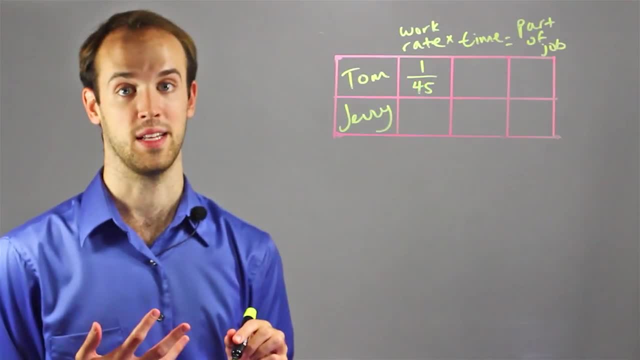 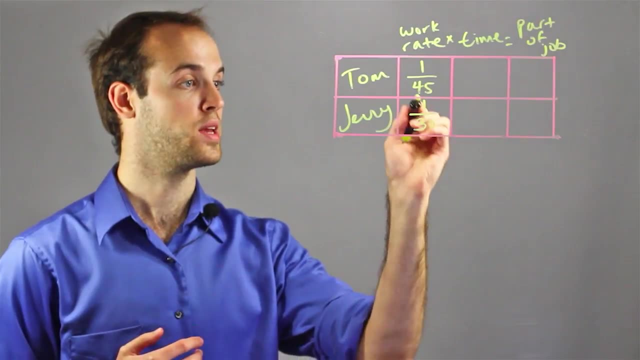 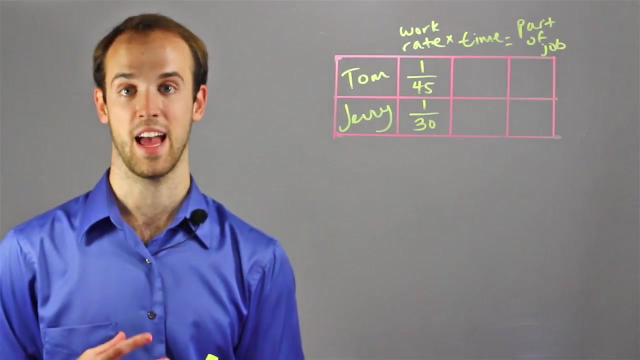 One car per every 45 minutes. Per usually means divided by. Jerry goes faster and he can do one car in every 30 minutes, So he's 1 over 30. The time is the unknown, because I want to know how fast it takes them washing the same car together. 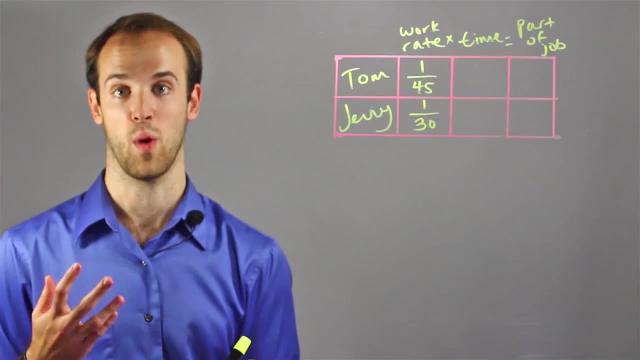 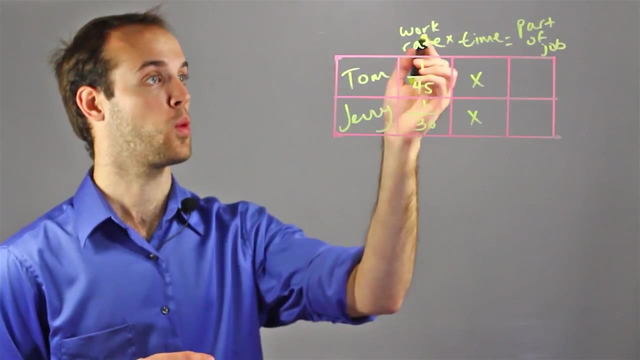 And they're going to work the same amount of time. It's not like Jerry's going to quit halfway through the job. They're both going to be represented by X And since I know that work rate times, time equals the part of the job. 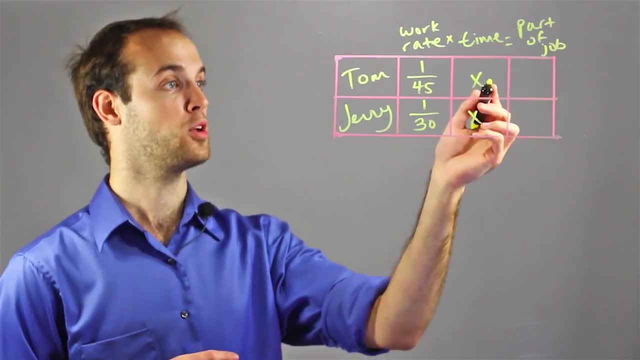 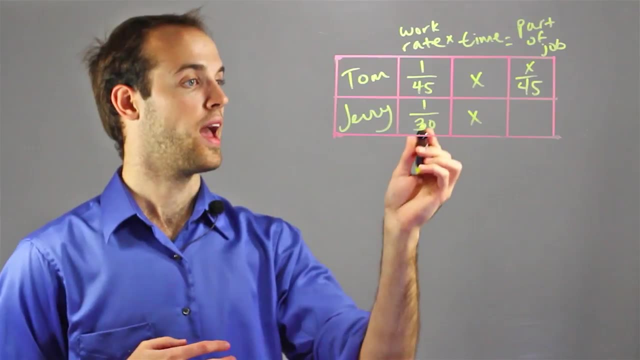 I know that I can get the part of the job column just by multiplying these two together. So X times 1 over 45.. 45 is equal to X over 45. And X times 1 over 30 is equal to X over 30.. 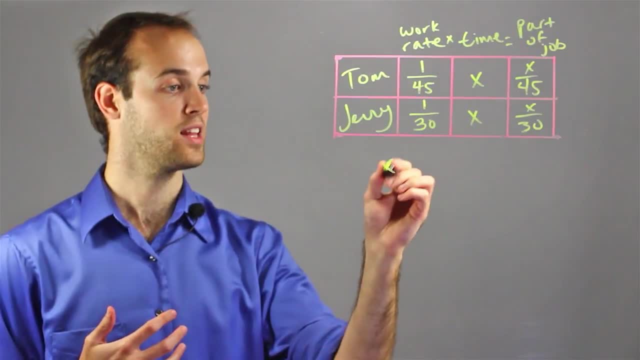 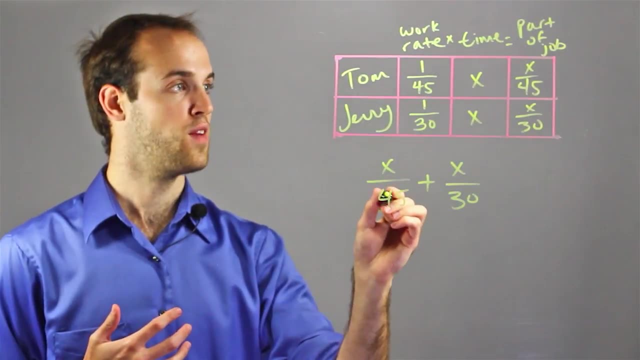 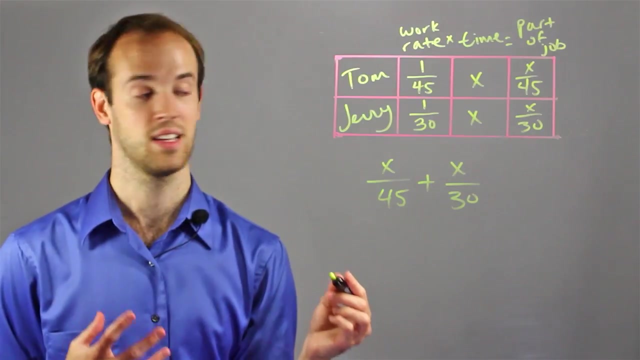 And now I'm ready to set up my equation, And I can get that just by adding the two parts of the job completed together, So X over 45, the part of the job that Tom completes plus X over 30, the part of the job that Jerry completes. 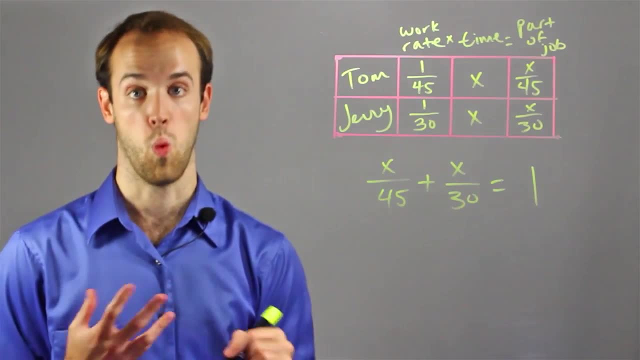 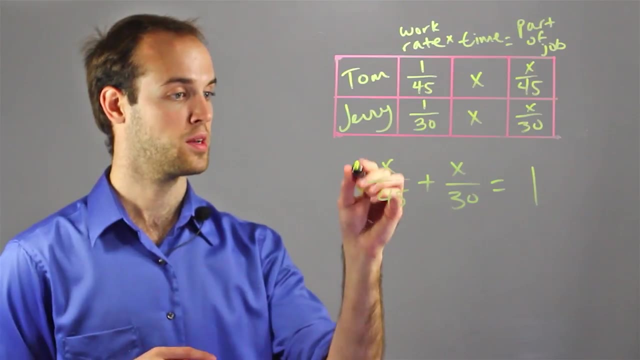 needs to be equal to 1.. 1 job: 1 job completed- 1 total job completed by both of them. So now I just have to solve this equation for X. The first thing I'm going to do is multiply both sides by 90,. 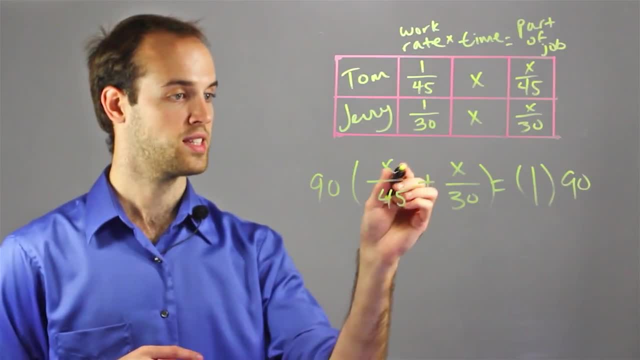 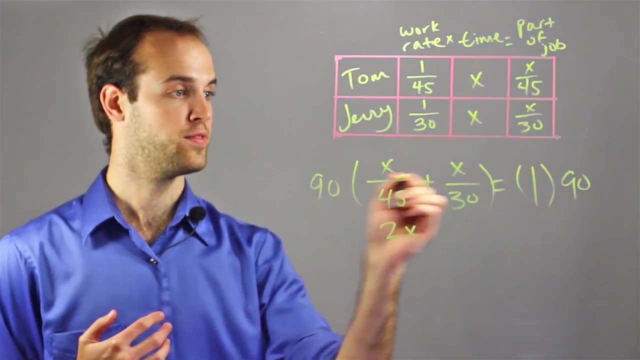 because that will get rid of all my fractions. So on this side I would have 90X over 45,, which would simplify to 2X, And in this term I'm going to have 90 times X over 30,, which is going to simplify to 3X. 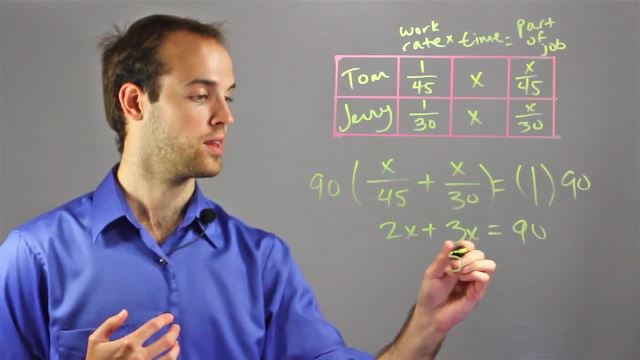 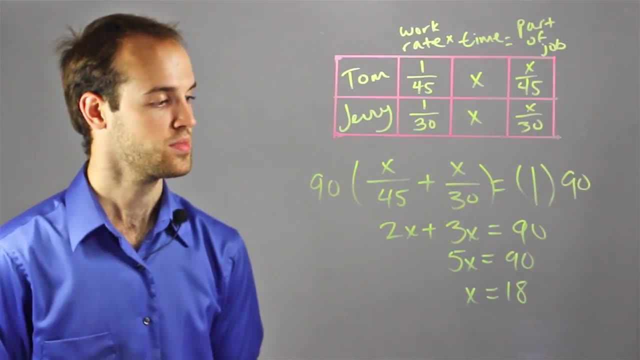 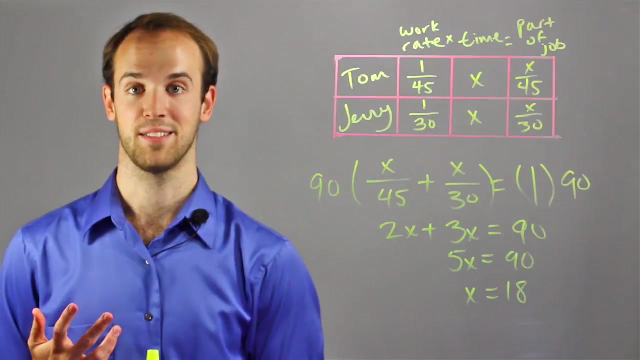 And that equals 90 times 1,, which is 90. And then combine like terms: I have 5X equals 90. And then divide both sides by 5, and I have X equals 18.. So I can now determine that, Tom and Jerry, if working together will wash one car in 18 minutes. 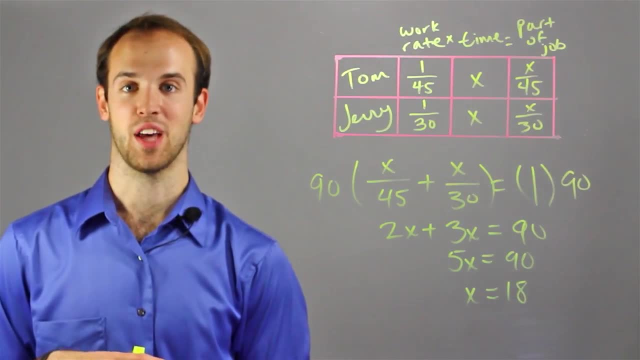 So I'm Drew Moyer, and this is the use of rational expressions in math in everyday life.